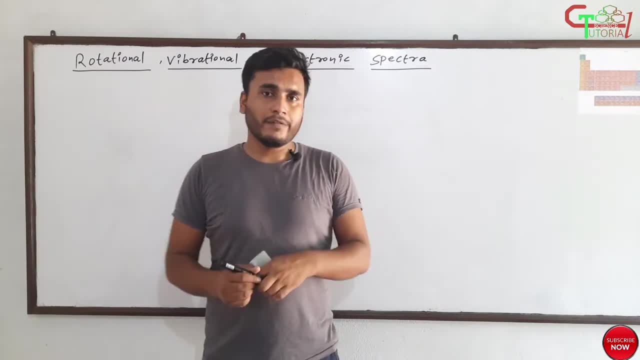 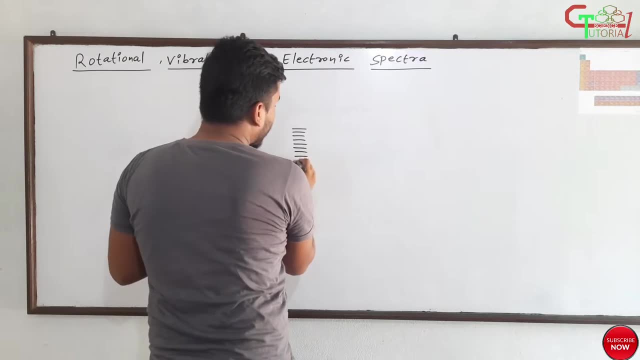 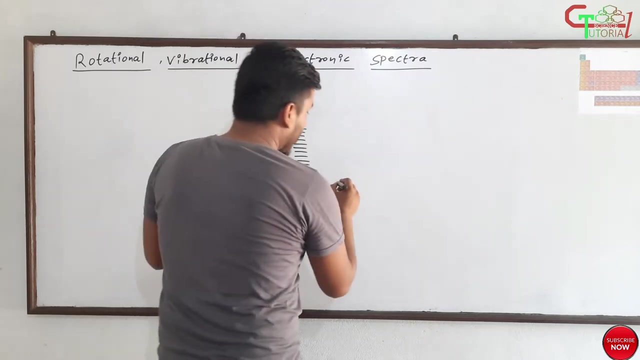 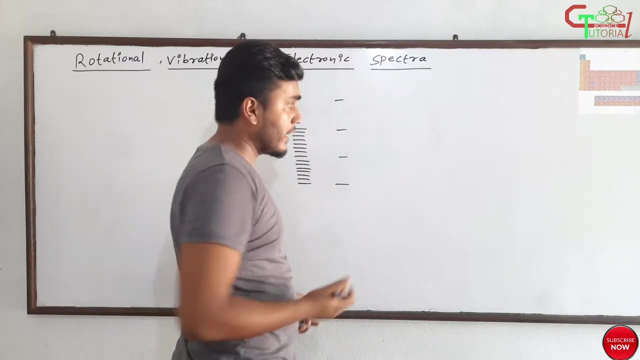 gap between those sets of energy levels are also different, Like this: some set might have energy gap very less and the spectra might be very close to each other, like this: Okay, this is one type of energy level. Another might be little far from each other. That means their energy gap might be little greater, and similarly, 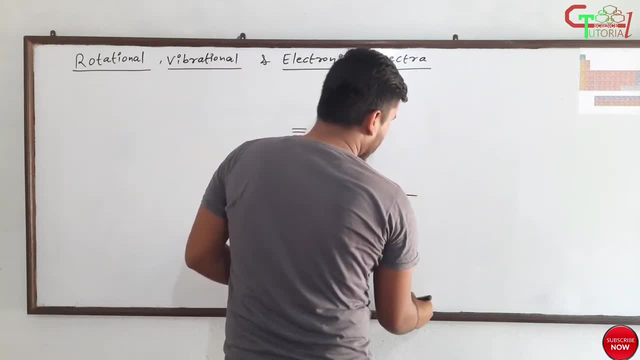 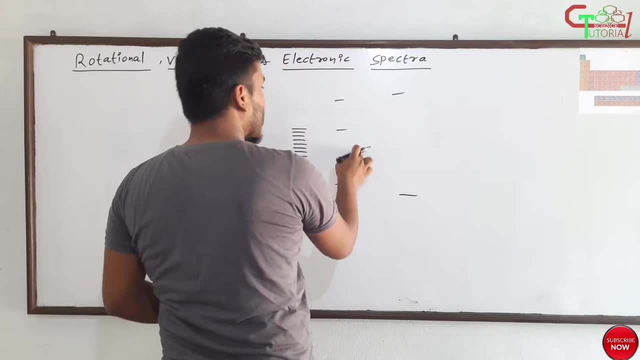 third one: their energy gap might be even more bigger, larger like this, Okay, like this. This is the first energy level. This is the second one Here in this particular case. first, second, third, fourth Here in this case, there you can see, first, second. 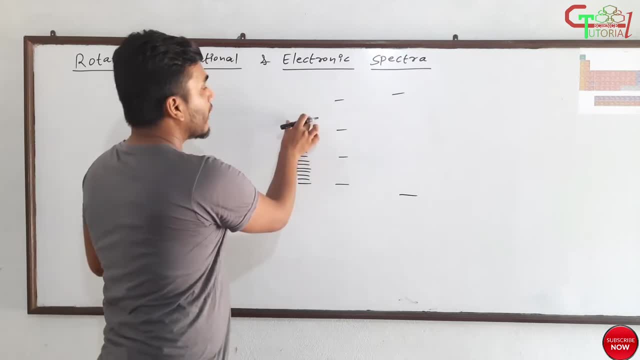 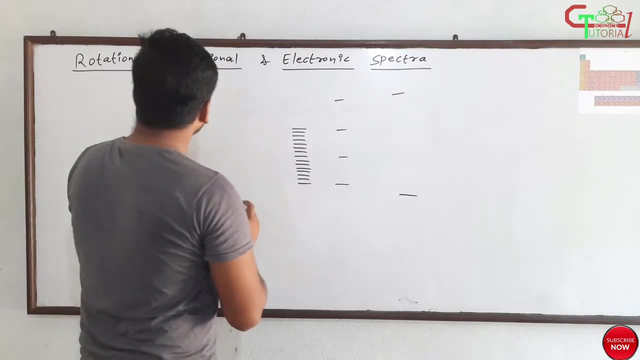 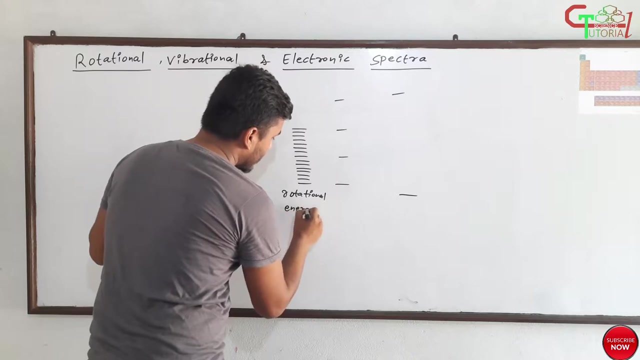 third, fourth, fifth, like that. Okay, now the energy level in which the energy gap is very less, Okay, in which the energy gap is very less, are called spectroscopy. Now, the second level is called rotational energy levels. Rotational energy levels. 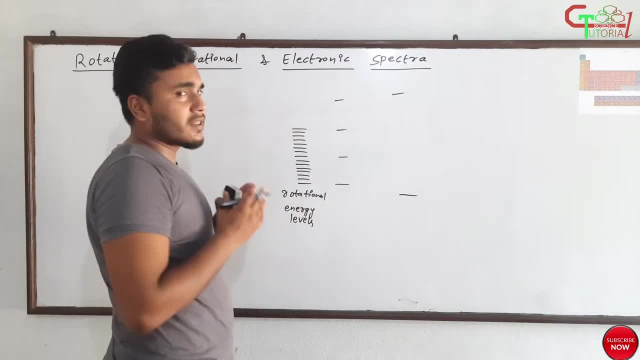 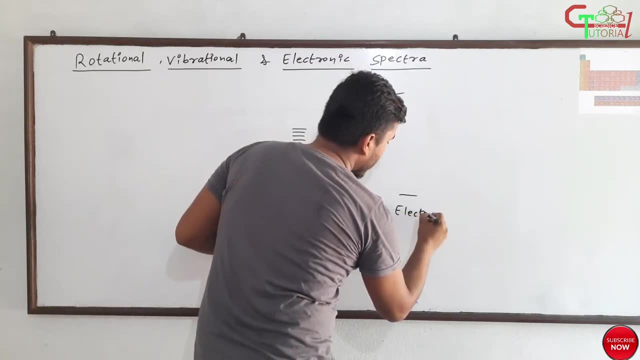 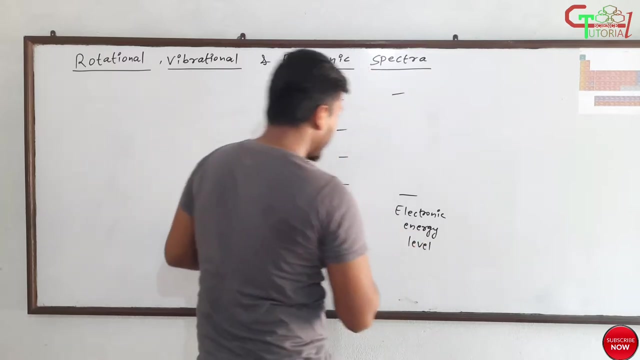 And the energy levels in which the energy gap is extremely large, that is maximum, is called electronic energy level, electronic energy level. Similarly, the energy level which is more than a pharmacy, which is more than a vitamin, is extremely large. Okay, and then when we compare the number between theكல referred to byล to next in here as обнаруж ladies'. 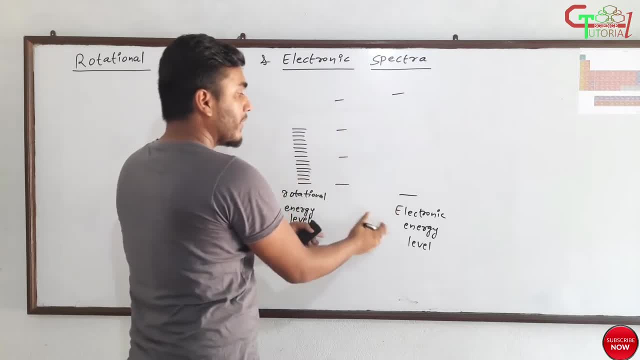 ordummalz구나 Esto mein energy labelwechsel. The negative energy level in which the energy rodeальный steeds and over the capitals in the hemisphere so that don't cause any significant level that is within them, between them. it's called vibrational energy level. 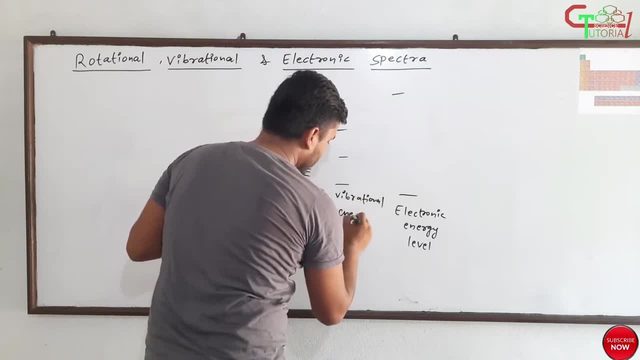 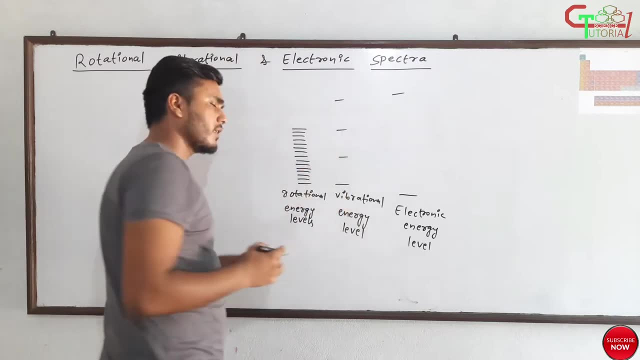 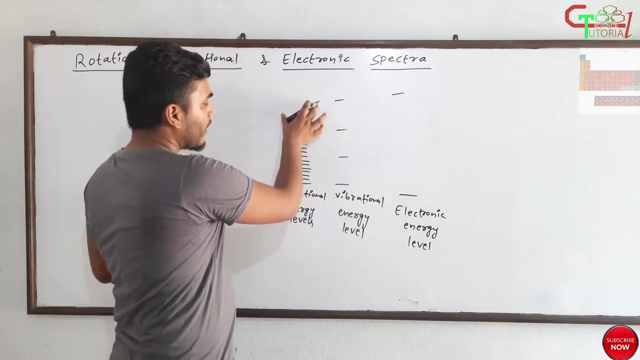 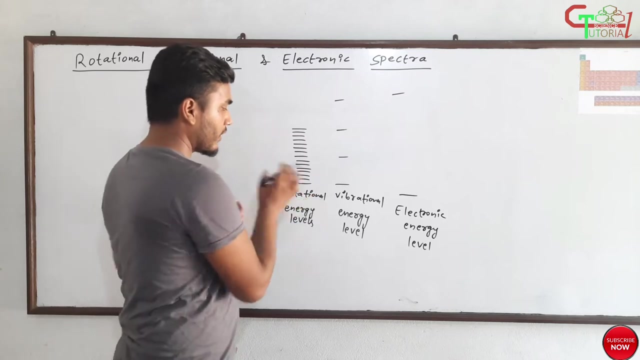 vibrational energy level. vibrational energy level, its energy, is somewhere between these two gaps. okay, the embrace bit of these and these. you can say that. so this type of energy levels, in which the energy gap between the energy levels is very least, are called rotational energy levels. and if the energy 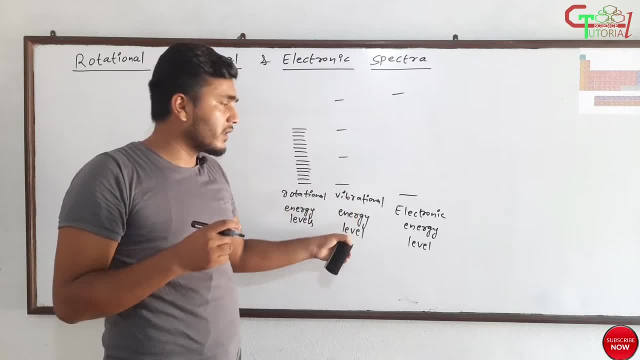 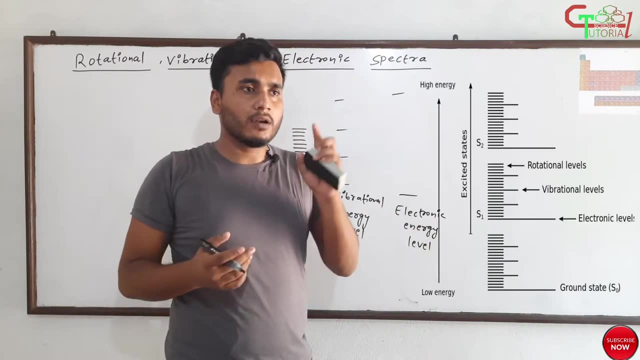 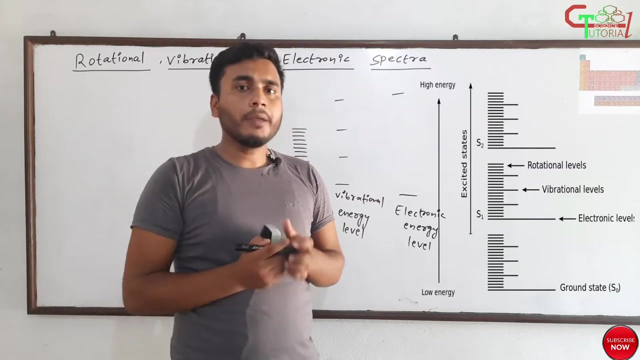 difference is little more. that is called vibrational energy level, and the energy gap is extremely large are called electronic energy level. you can see a picture on the display as well. you can see the concept over there how the energy levels are distributed. okay, now let's understand what's a rotational 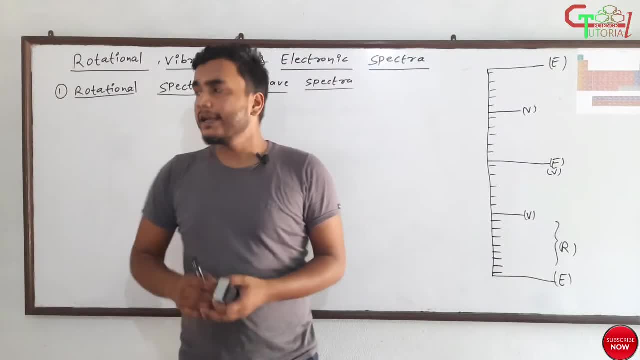 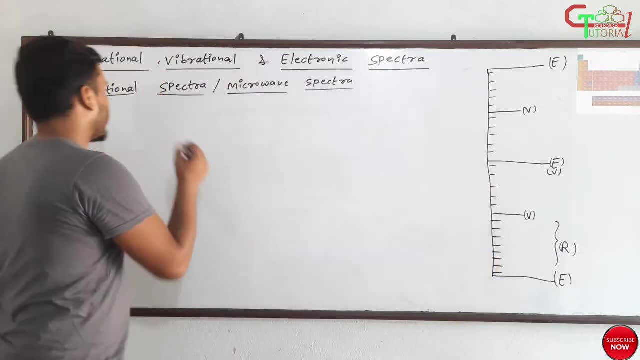 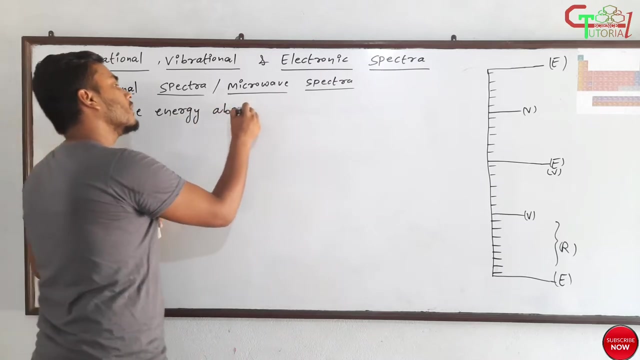 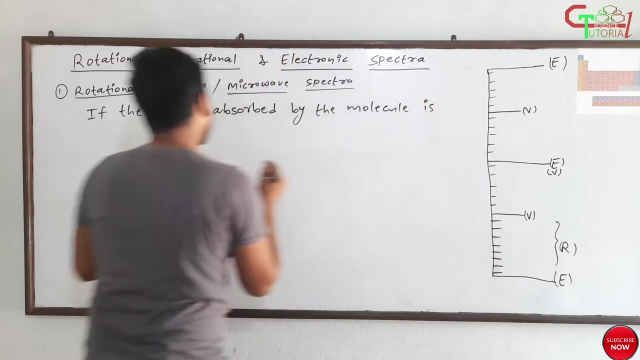 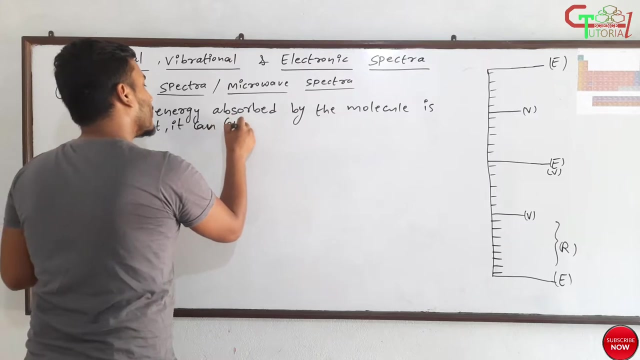 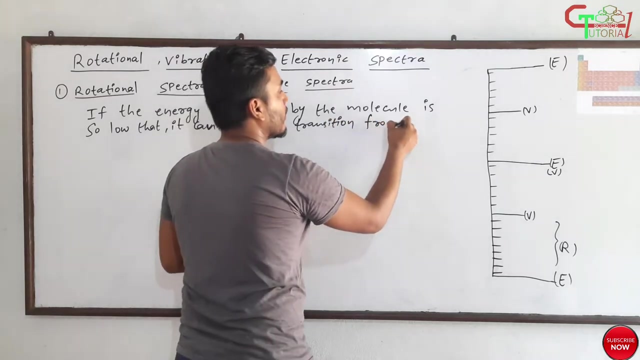 spectra actually are. first of all, let's understand about rotational spectra. that is also called microwave spectra. let me write the theory of it. if the energy absorbed, if the energy absorbed by the molecule, by the molecule, is so low that that it can cause, it can cause the transition that you can call the transition from one one rotational. 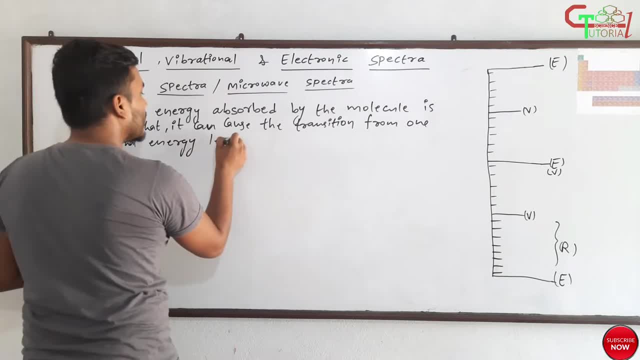 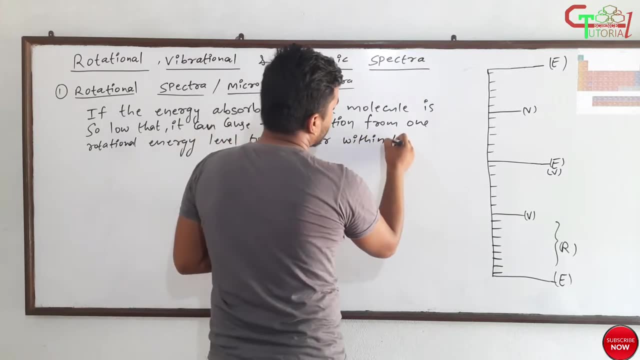 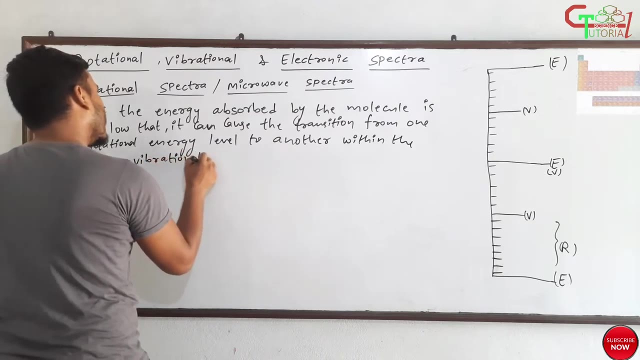 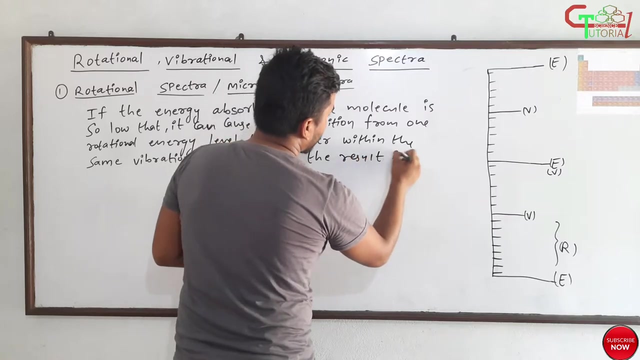 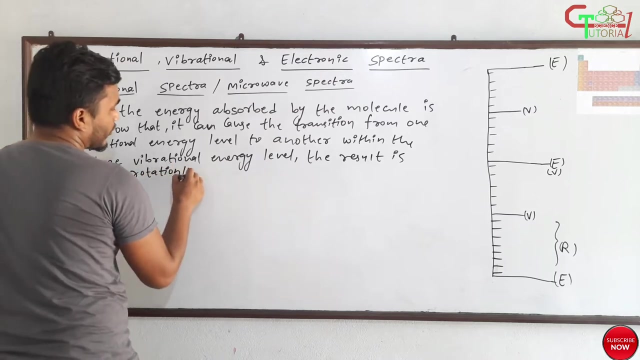 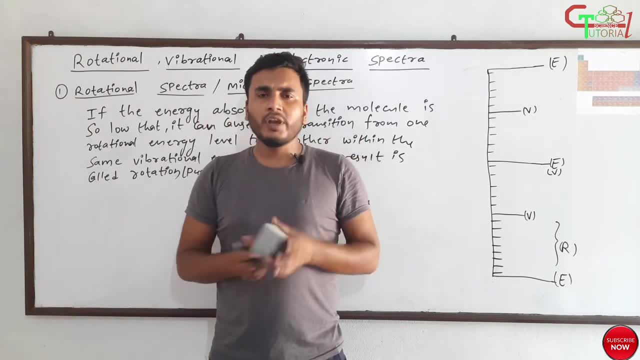 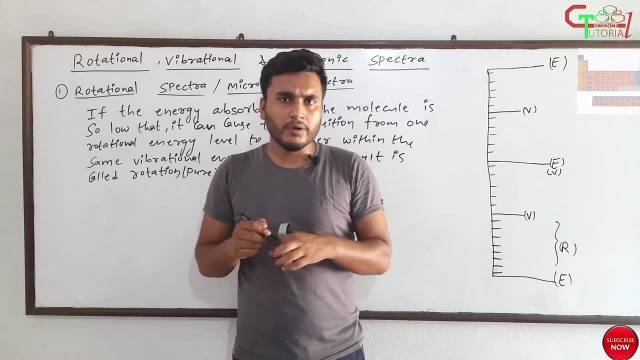 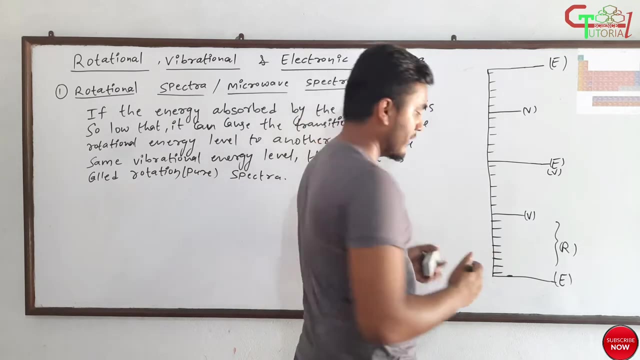 sometimes the molecule can absorb only very less amount of energy, and if it gets less amount of energy, then the transition will also be very small, right? suppose the molecule is over here now, right now, okay, in ground state. now it absorbs some of the energy and it will now make graph like this, that is, it is. 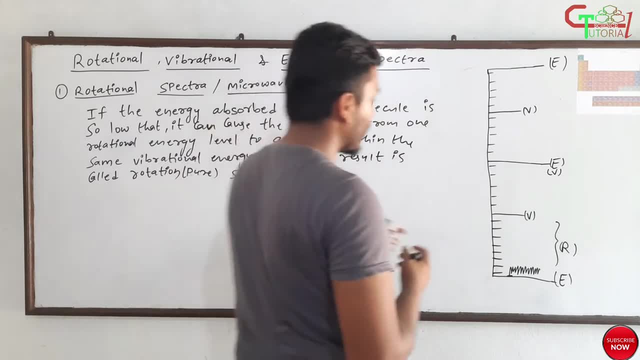 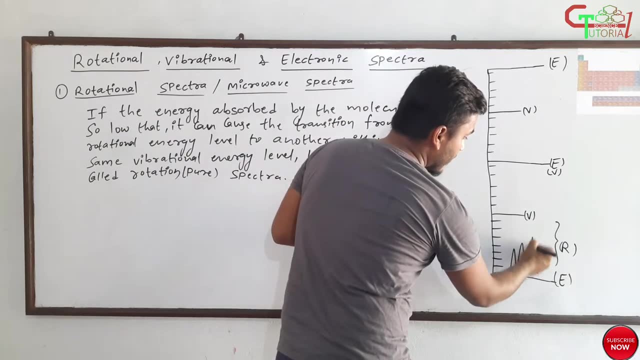 being like the transition is occurring only among some of the rotational energy, from one rotational energy to another. it can be like this as well: right now, these are all rotational energy level, so the transition can occur within this line. ok, within these lines, okay, within these lines. okay within these lines, okay, within. 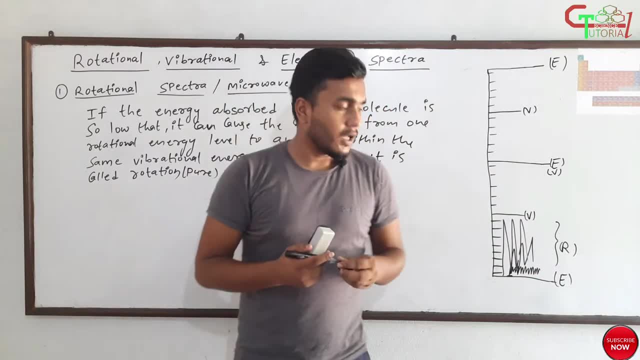 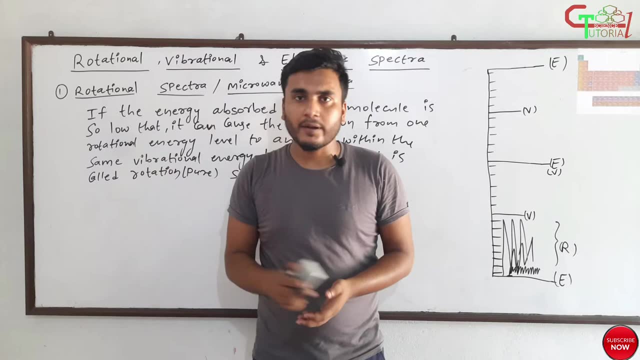 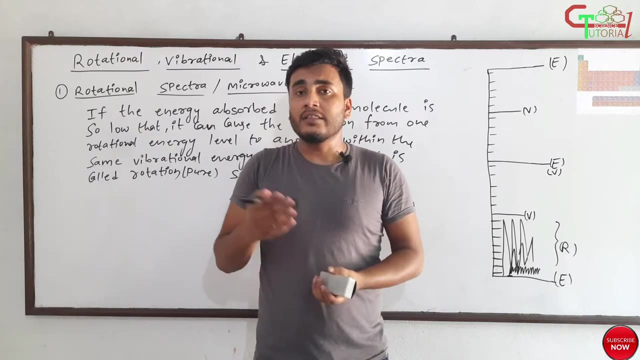 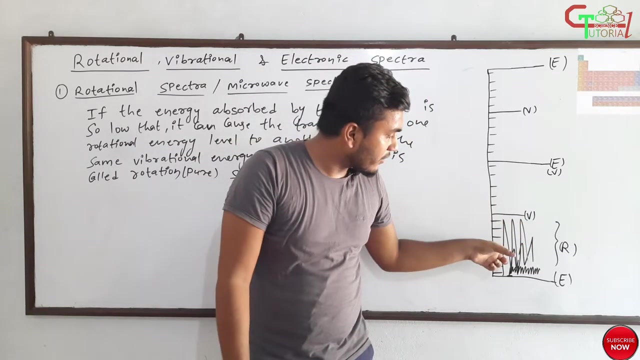 this line anywhere from anywhere. suppose the molecule is at this position, then if it transits to this one, then also it is called rotational spectra because the transition is happening within the rotational energy level right now. so as long as the transition is occurring within the rotational energy levels, within the same vibrational energy, right now it is being 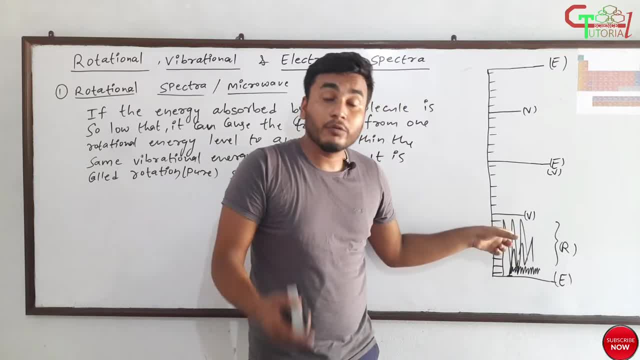 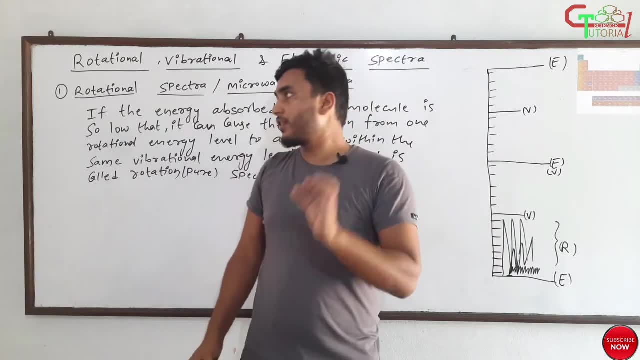 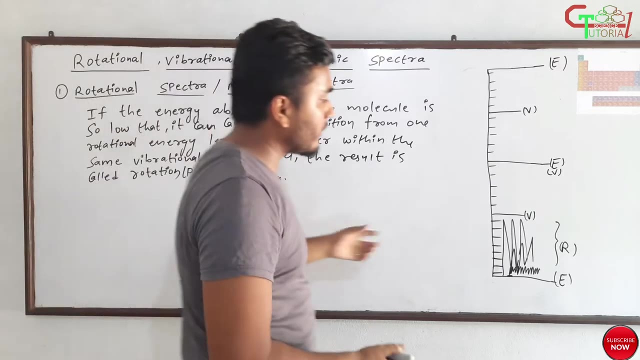 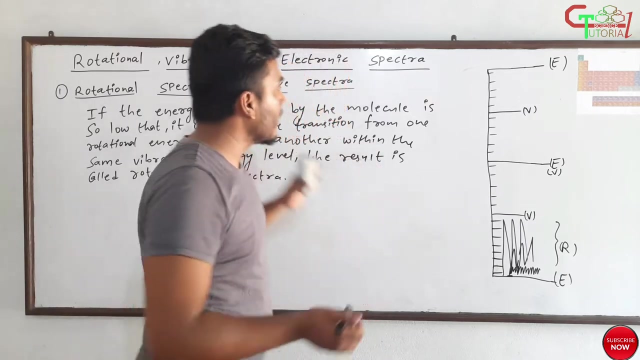 transitioned from one rotational energy to rotational energy, to another rotational energy within the same vibrational energy, right? so this type of result is called rotational spectra, and this is also called microwave spectra, as the wavelength of the radiation is within microwave- okay, within microwave region. that's why it is also called microwave spectra. now let's understand. 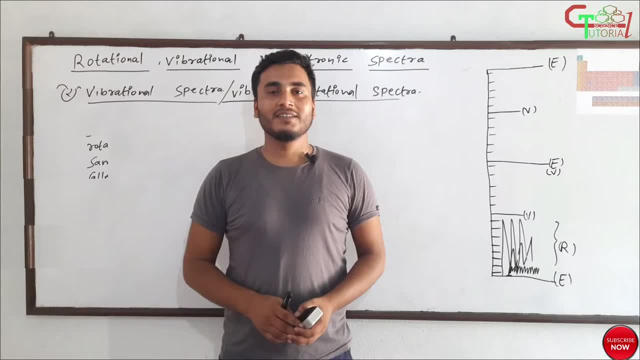 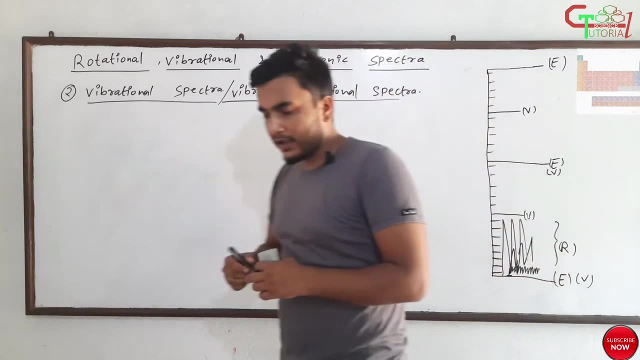 what vibrational spectra. so let's understand what vibrational spectra is. so let's understand what vibrational spectra is actually is. now let's understand about vibrational spectra that is also called vibrational rotational spectra. let me write the theory of it and it will be very easy for us to. 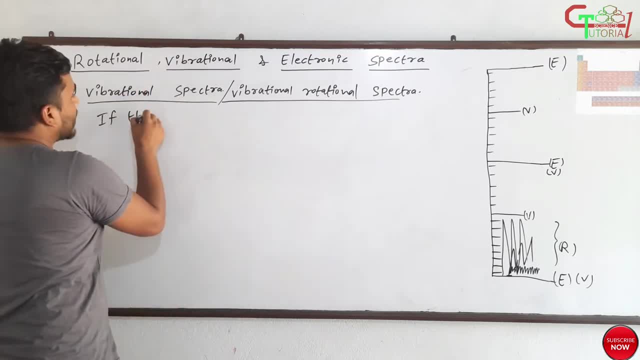 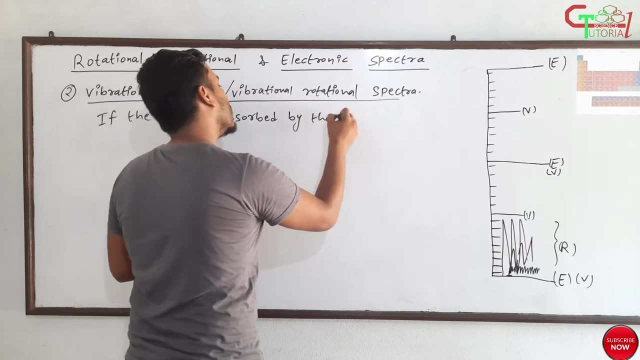 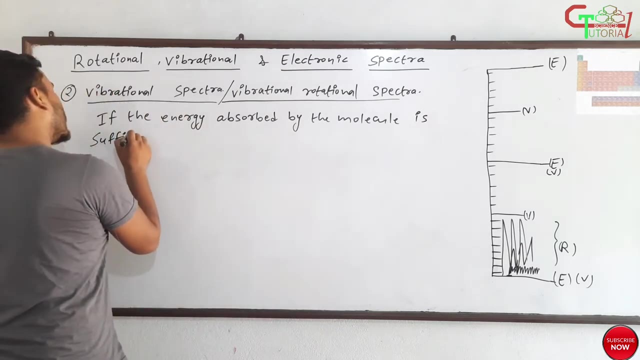 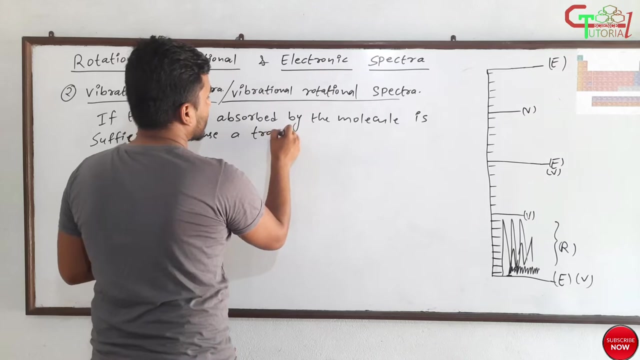 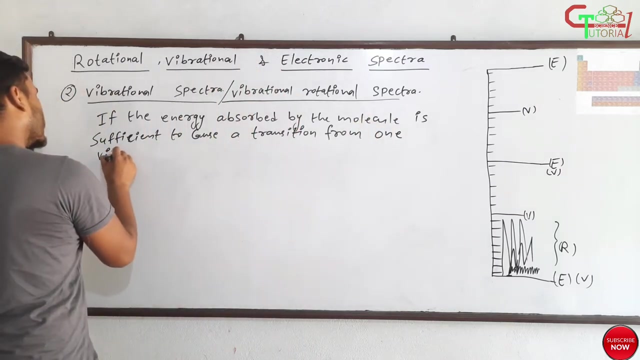 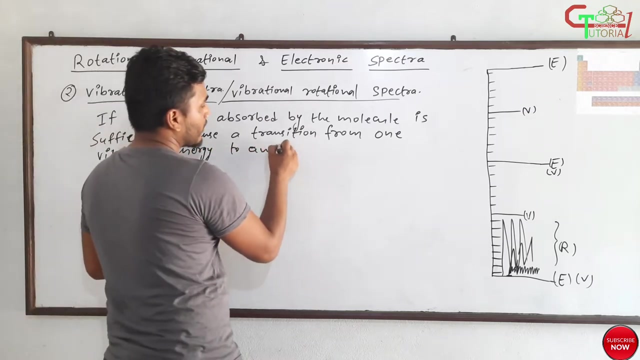 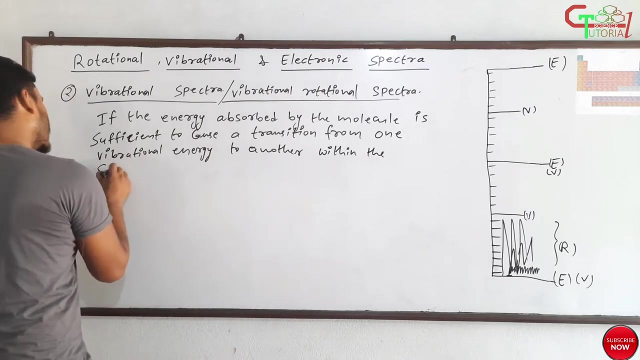 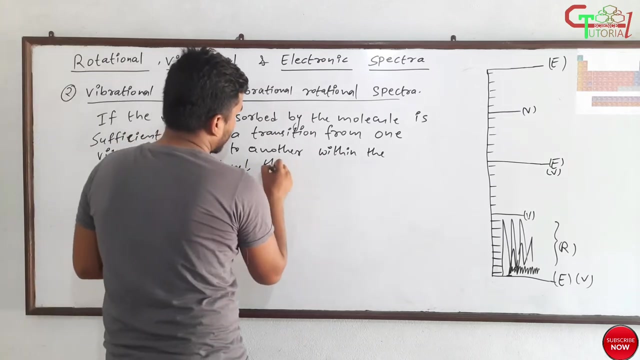 understand it, if the, if the energy absorbed by the molecule, by the molecule, is sufficient sufficient sufficient sufficient sufficient to cause, to cause a transition, to cause a transition from one vibrational energy to another another, within the, within the same same, within the same electronic level. electronic level, the result, the result. 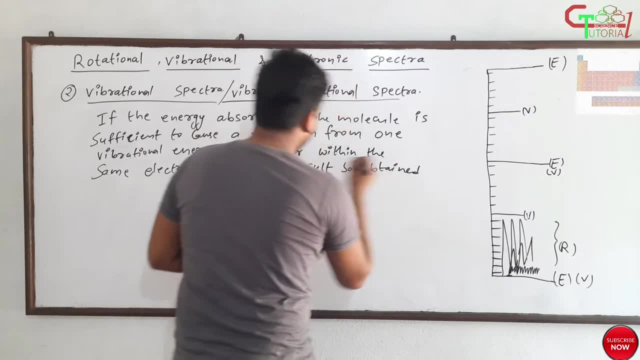 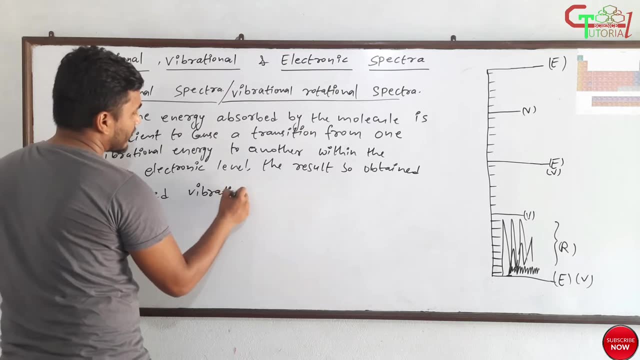 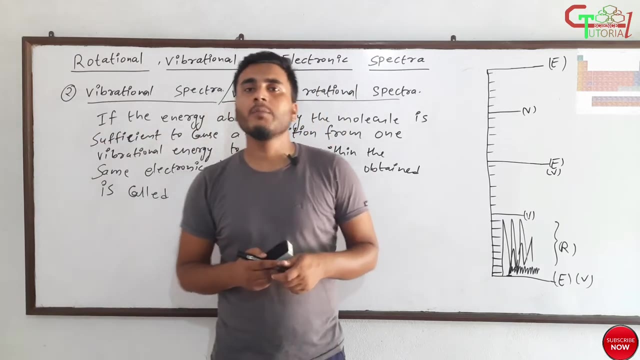 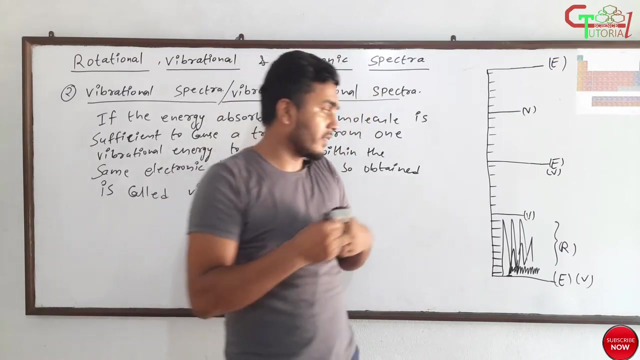 so obtained. the result so obtained is called vibrational vibrational spectra spectra. now, this theory is trying to say that sometime the molecule can absorb a little more amount of energy, and if that gets a sufficient amount of energy, then the transition might occur from one vibrational energy to another vibrational. 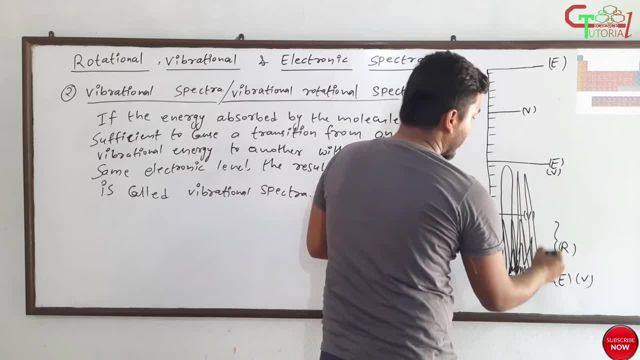 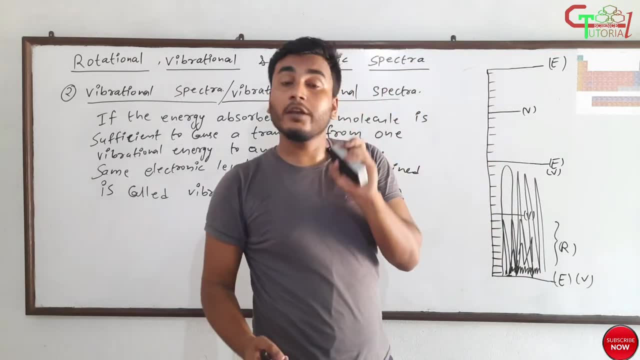 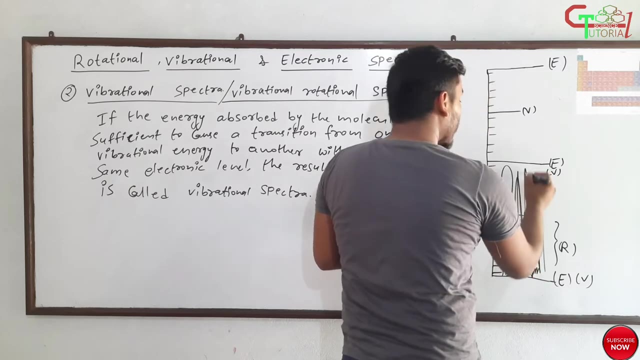 energy like this: okay, it can cross one vibrational energy, but that should be within the two electronic spectra. okay, in the electronic energy levels from here to here and then either here to here. so the yes, the spectra will have a sufficient energy in that scenario, amount of energy that is, it will show vibrational energy it will cross. 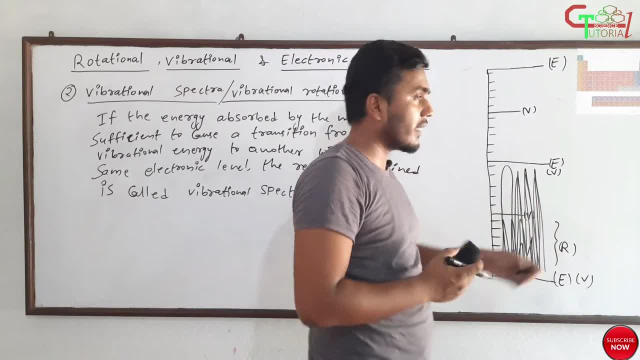 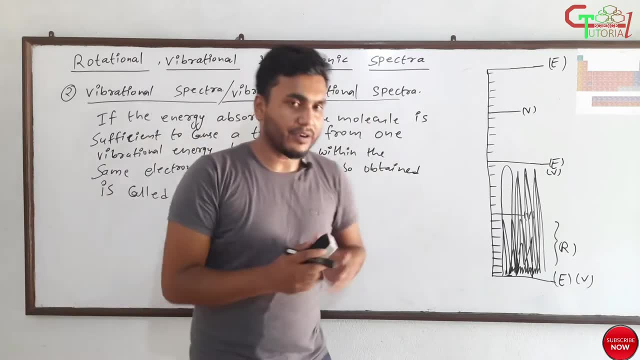 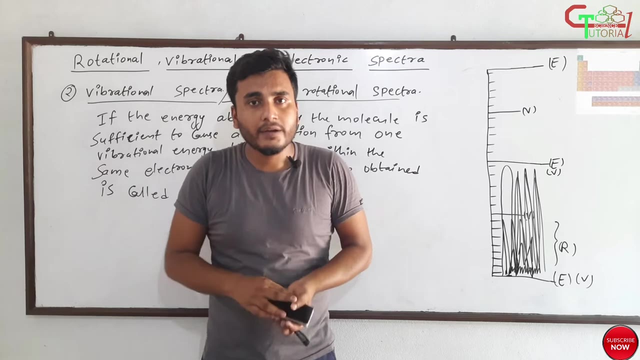 vibrational energy level, but that should be within the electronic energy level. and if we get that type of spectra, then those spectra are called as vibrational spectra, and in that case the wavelength of the molecule might be each in infrared region. that's why it is also called infrared spectra. so the only 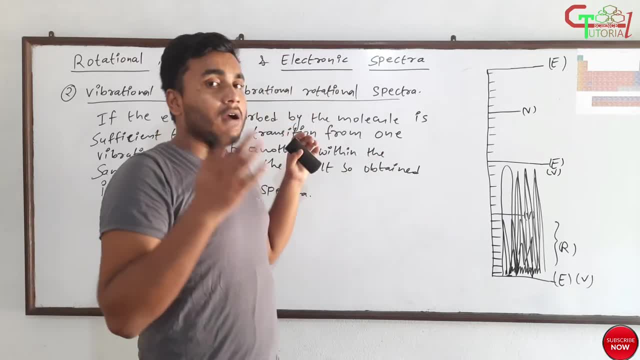 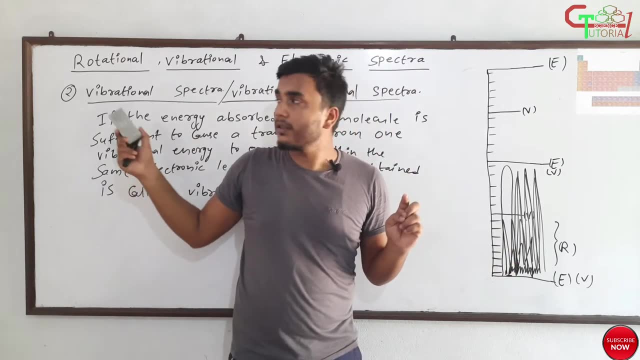 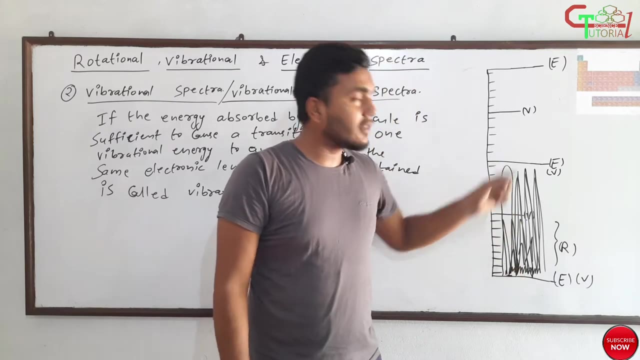 difference between that is, in that particular case, in rotational energy levels. the transition was only among the rotational energy levels, but in this particular case, that is in vibrational energy level. you can see over here, the transition is from one in a vibrational energy level to another vibrational. 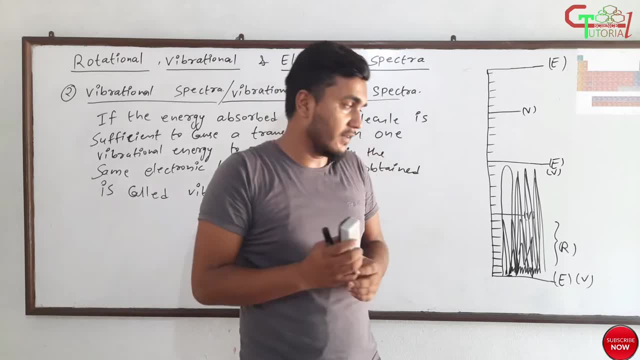 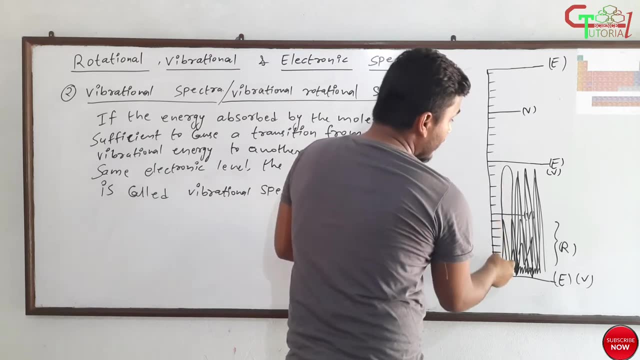 energy level. okay, but that should be within two electronic energy levels. and in this particular case you can see over here if the molecule transits from over here to here. it is not only. you can see over here. if a molecule transits from over here to here, it is not only. 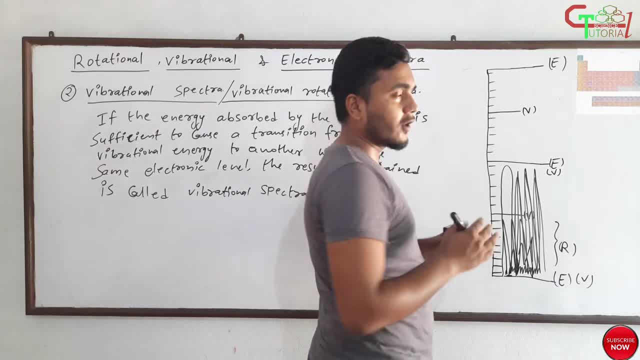 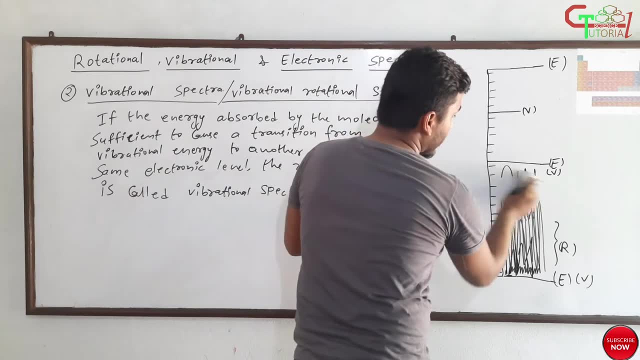 being transitioned from one vibrational energy to another vibrational energy, being transitioned from one vibrational energy to another vibrational energy, but it is also being transition from one rotational energy to another rotational energy. like this. let me read this part like this, from here to here: if it is happening like this, then 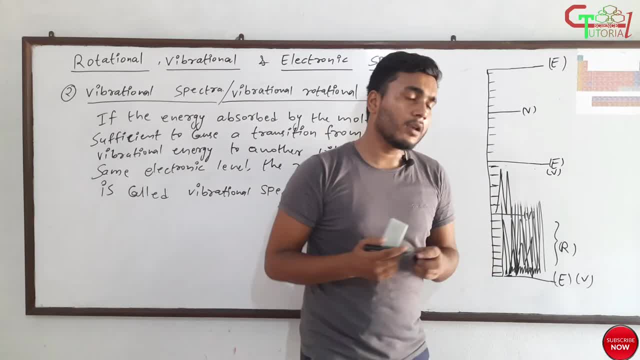 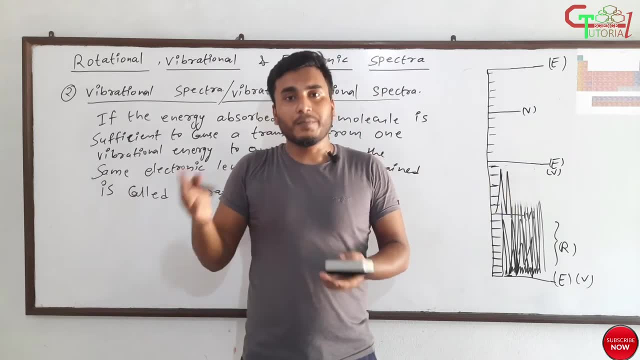 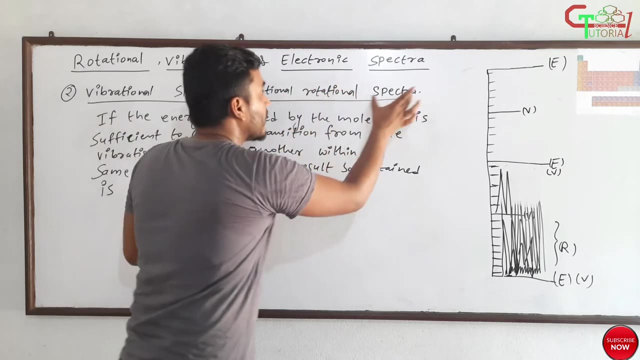 obviously from one rotational energy to another rotational energy also, it is being transitioned. so in this particular case there is not only vibrational vibrational spectra, but we get the rotational spectra as well, so that's why it is also called vibrational rotational spectra. now let's see the 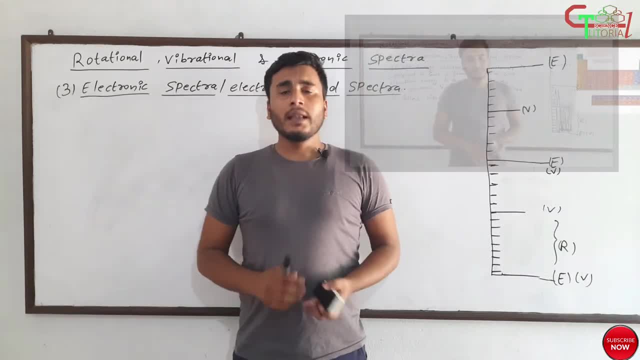 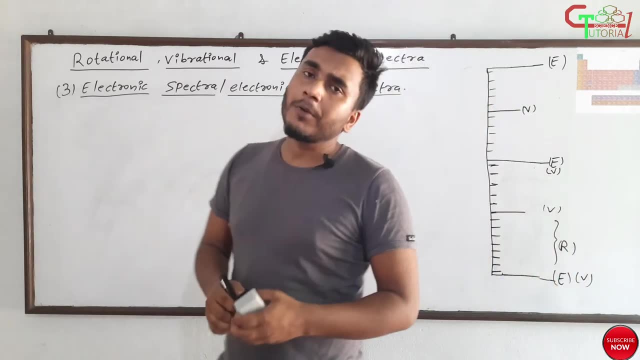 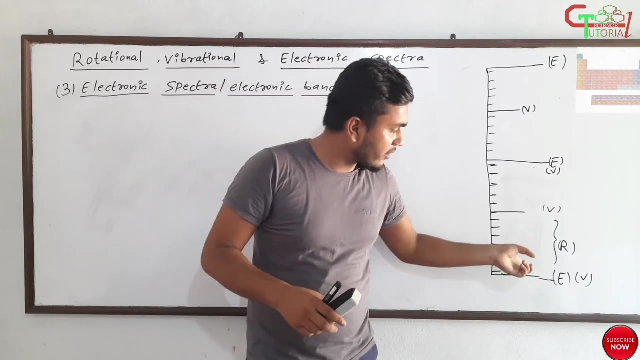 last one, that is, the electronic spectra. now the third one is electronic spectra, or that is also called electronic band spectra. in this particular case the exciting energy is extremely high that the transition can occur from one energy level, electronic energy level, from another, electronic energy level. let's 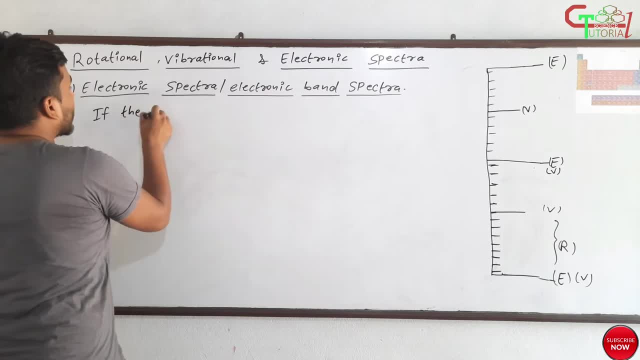 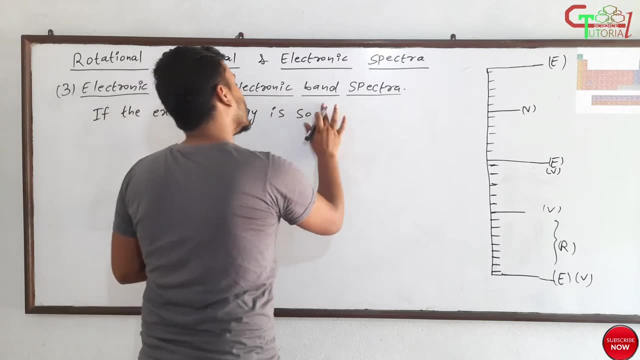 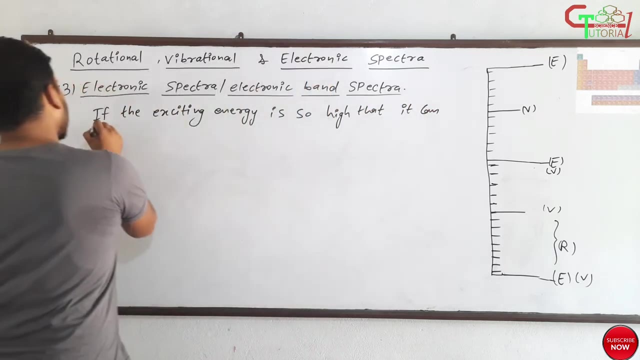 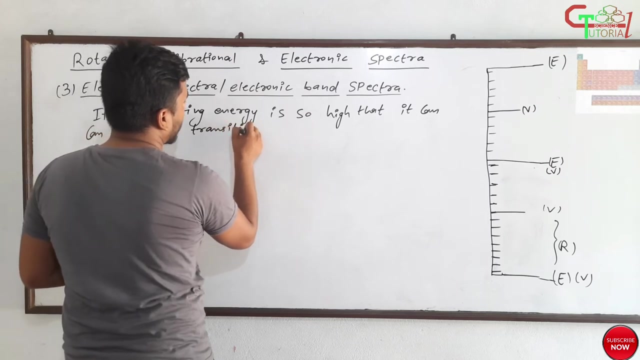 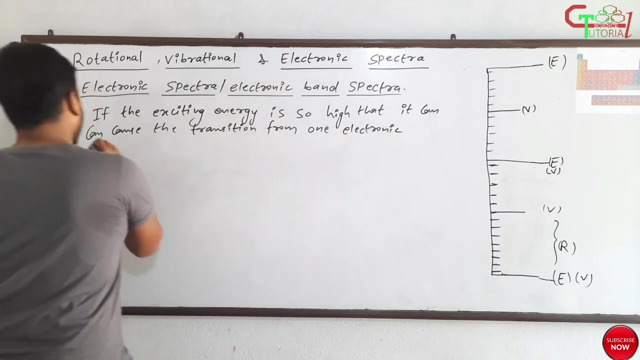 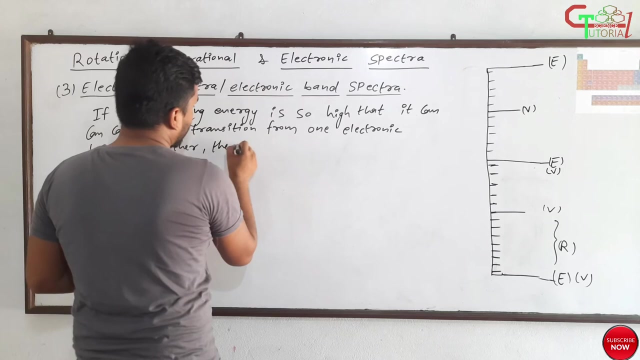 write the theory of it. if, if the exciting energy is so high, see if, if the excited energy is so high, it's so high that it can cause that. it can cause the transition. it can cause the transition from one one electronic level, or simply energy level, to another, to another. the result: the result obtained.